Your heart pumps the blood up to your brain Without gravity, pulling blood down into your legs and feet. more blood would stay in the chest and head. This is why astronauts have puffy faces, And having extra blood in the brain makes the body think that there is too much blood. After only a few days in space, the astronauts' bodies make less blood- Around 20% less- And with less blood to pump, the heart muscle also shrinks. Oh, I made the simulation too big. Without gravity, everything from the atmosphere to the water in the ocean, to animals and soil. 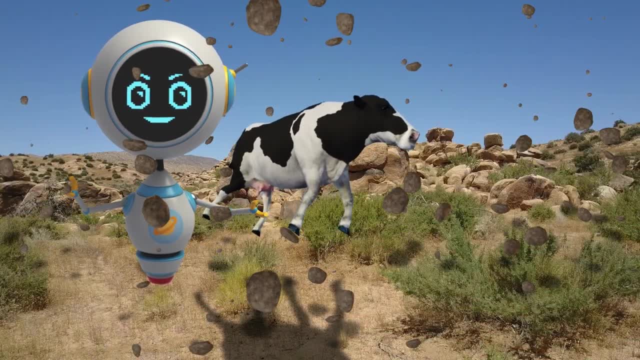 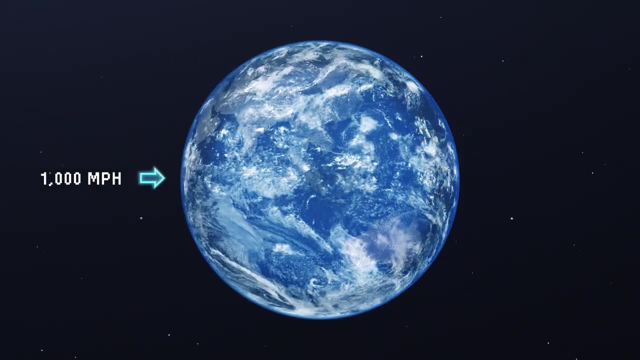 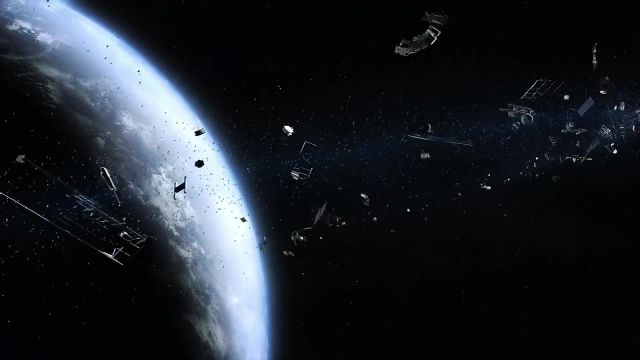 will float away. Maybe float isn't the right word. With the Earth still spinning at its usual 1,000 miles per hour, everything that isn't attached to the ground would go flying At the equator, where Earth spins the fastest. 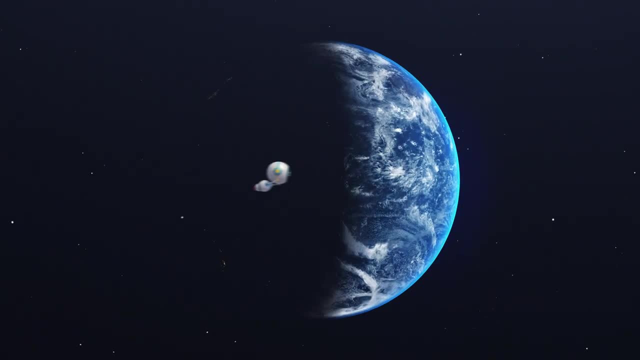 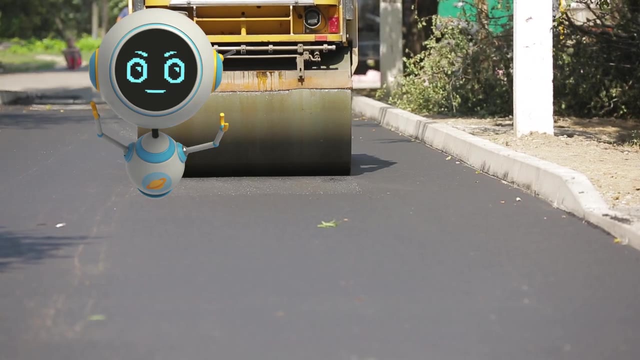 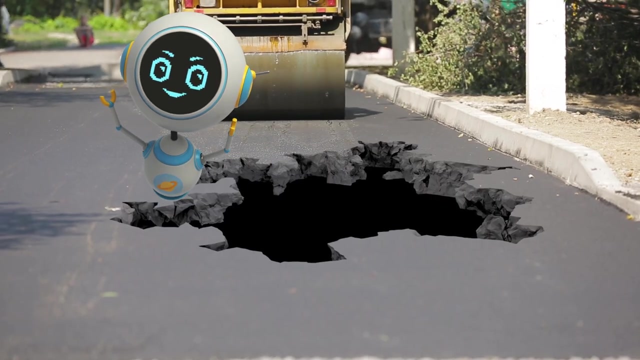 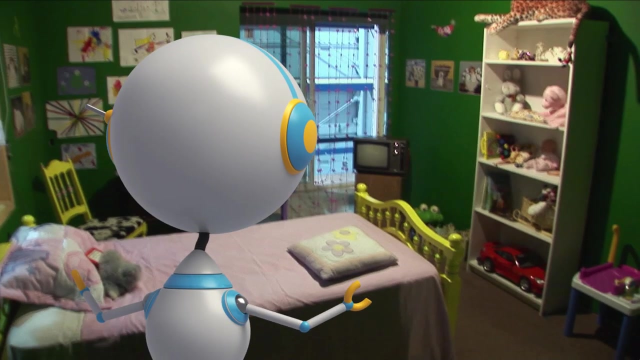 you would be blown as far as 1.4 miles in just five seconds. Whee Oops. The Earth is kept together by gravity. If gravity disappeared, the pressure of the Earth's core would cause the Earth to burst open. You would feel enormous earthquakes. 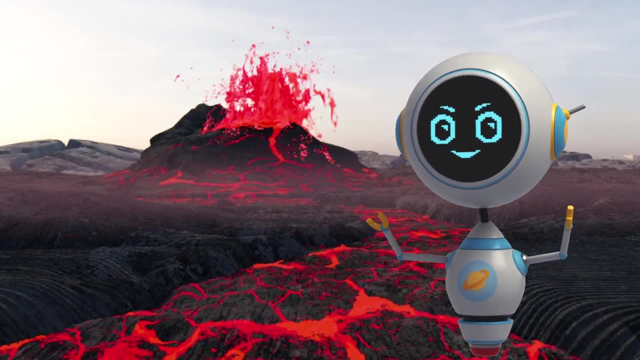 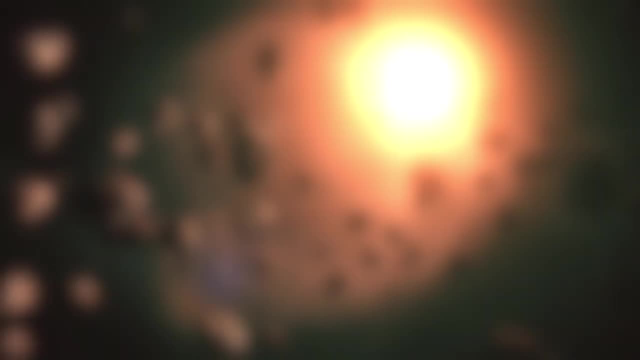 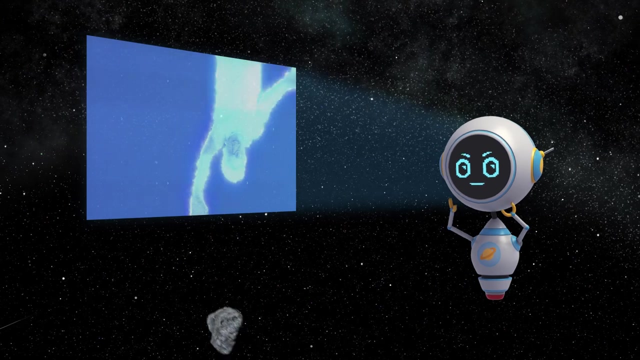 Gigantic volcanic eruptions would send lava floating in every direction. Eventually, the Earth would break into pieces that would then drift away into space. Put it back, Put gravity back. The astronauts I saw at the International Space Station said: The astronauts I saw at the International Space Station said: 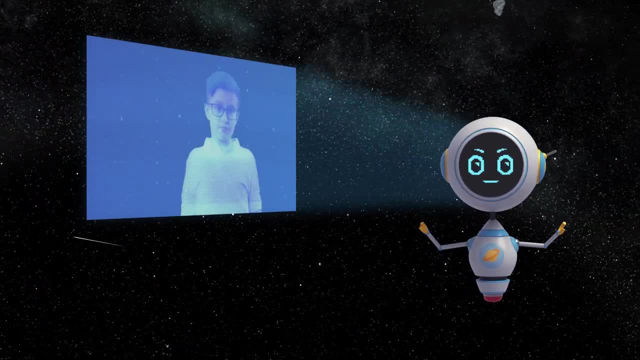 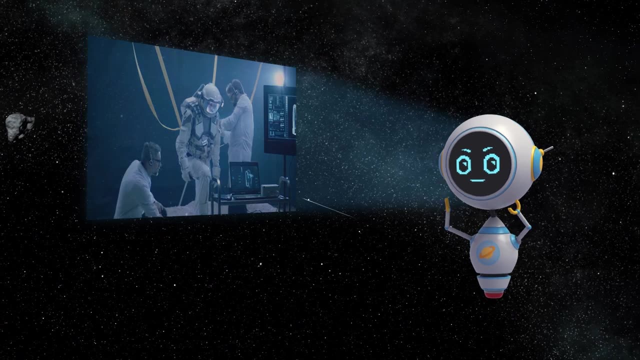 The astronauts I saw at the International Space Station said I thought the space station seemed so happy. I thought the space station seemed so happy. Why weren't they terrified? Astronauts train to work in an environment with no gravity. They wear special clothing to keep more blood in their legs. 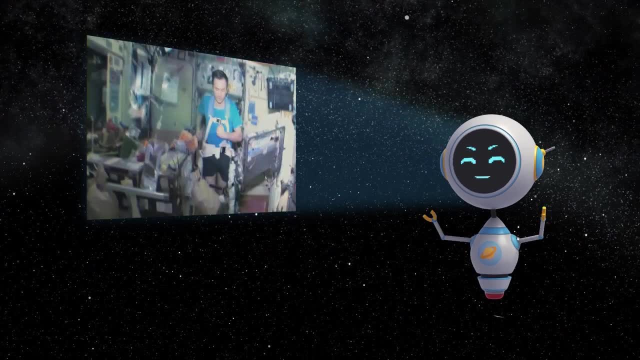 They exercise every day to keep their heart healthy. They exercise every day to keep their heart healthy, their bones and muscles strong. They exercise every day to keep their heart healthy, their bones and muscles strong. They even test their urine to check their health in space. 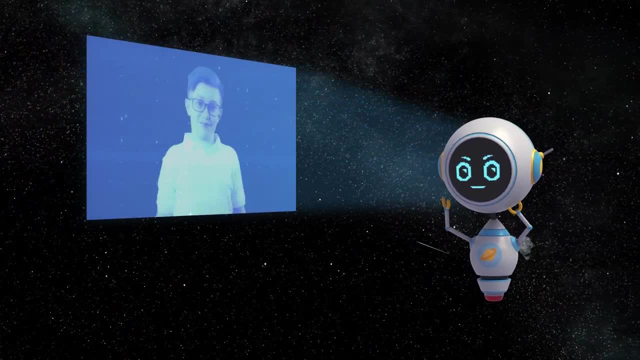 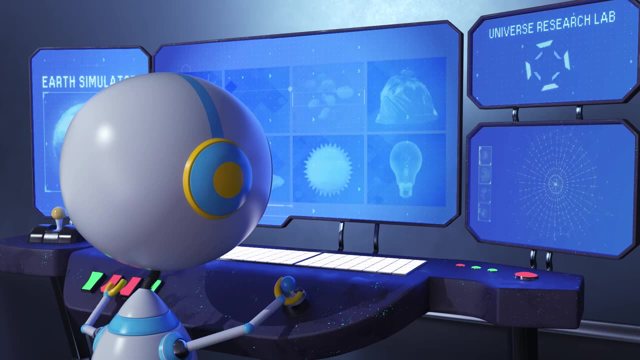 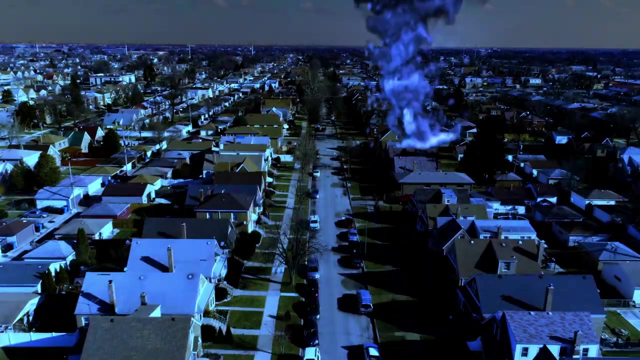 Maybe one day I'll see you in space Cosmo. Maybe one day I'll see you in space Cosmo. Bye, See you later. Hmm, which chapter should I research next? Cosmo, Hey everyone, Cosmo here. 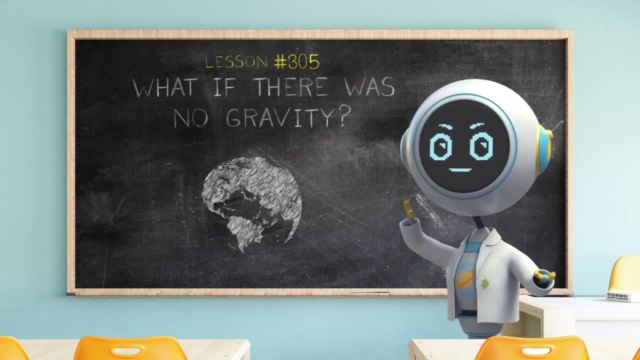 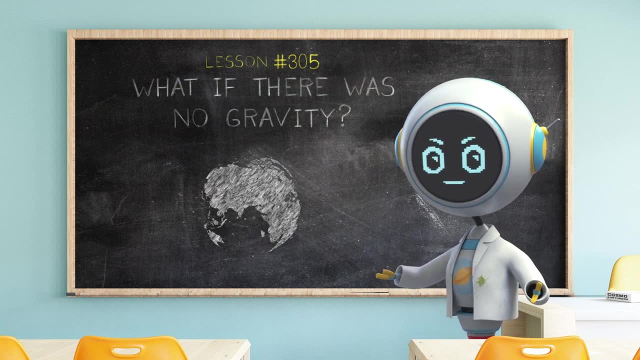 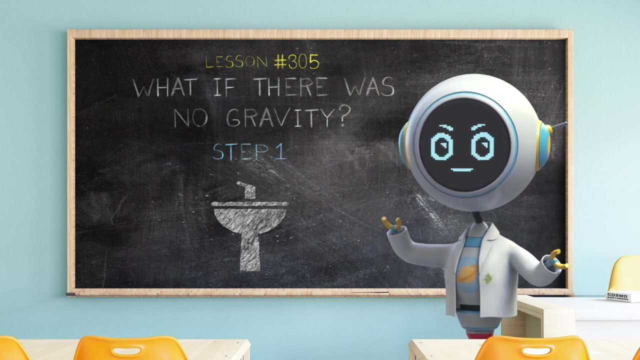 Luckily, gravity will always be with us on planet Earth. but what if you could do a magic trick that looks like you were defying gravity? This trick might get messy, so try it over the sink or a large bowl. Step 1. Gather your supplies.